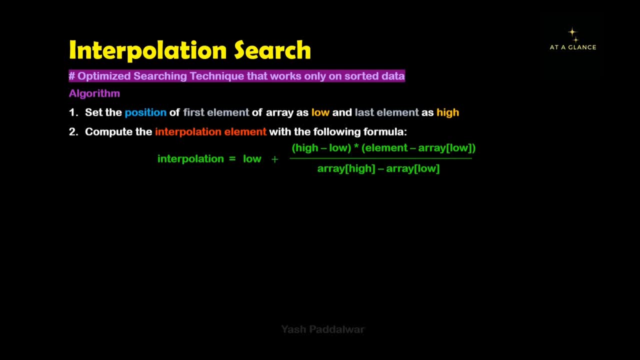 low, plus high, minus low, into element that is to be searched, minus the element which is located on the low position, divided by the difference between the element which is located on the high position and the element which is located at the low position. Now next step is to compare the element which is located on the interpolation position with the element to be searched. 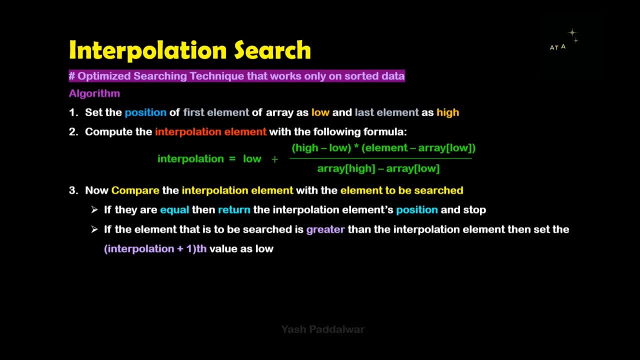 If both of them are equal, then you need to return the interpolation element's position and stop, because it is found Now. if the element to be searched is greater than the element which is present on the interpolation position, then you need to set low as high. 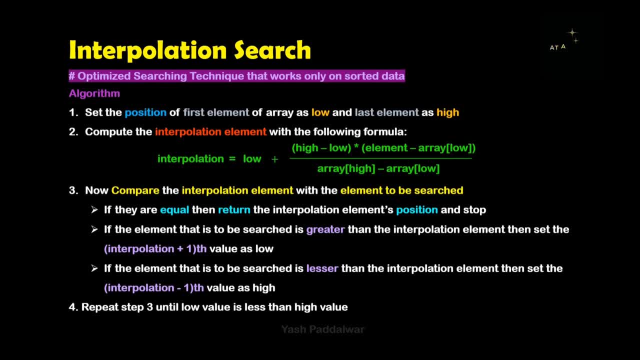 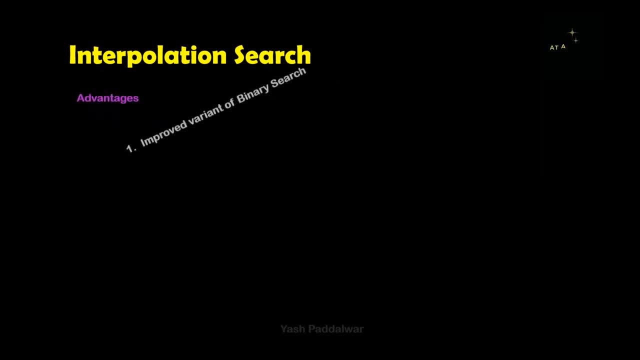 Interpolation plus one, otherwise set high as interpolation minus one. Finally, you will get the element to be searched. Now let's have a look at the advantages of interpolation search. First is that it is an improved variant of binary search, because it can find the element in single iteration if the data is uniformly distributed. 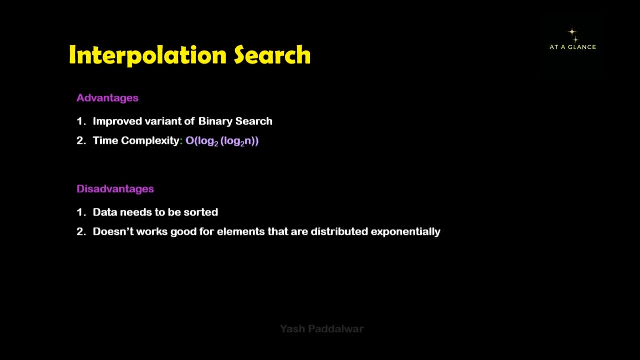 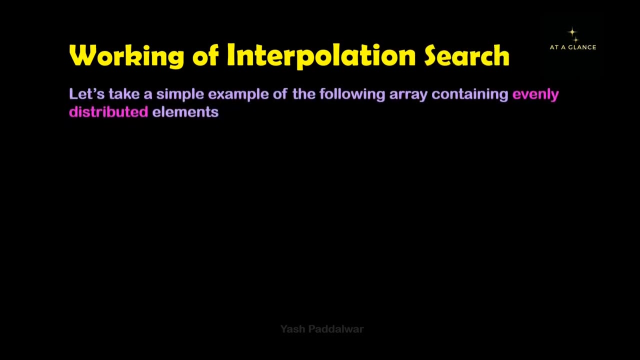 Its time. complexity is O Talking about the disadvantages. First, the data which it requires needs to be sorted, and it is not recommended to use interpolation search when the data is exponentially distributed. Now, with the help of example, I will explain you how interpolation search algorithm works. 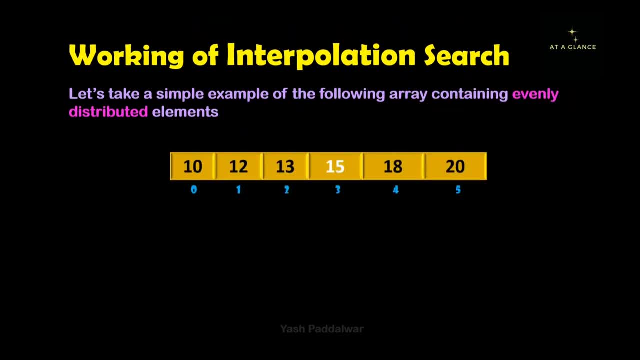 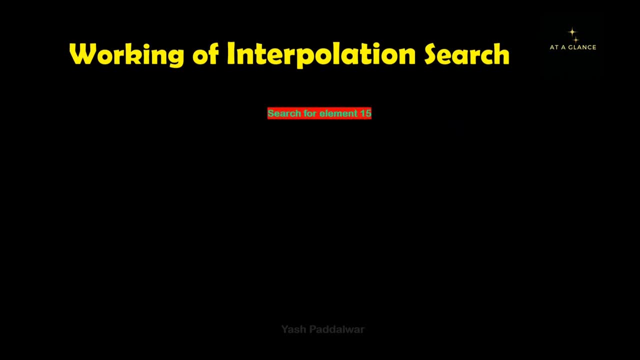 So that you will understand the entire working. Now, here we have taken an example of a sorted array. Let's find the element 15.. Now, as per the algorithm, the first step is to set the low and high values. Clearly, the low is the 0th index and high is the 5th index. 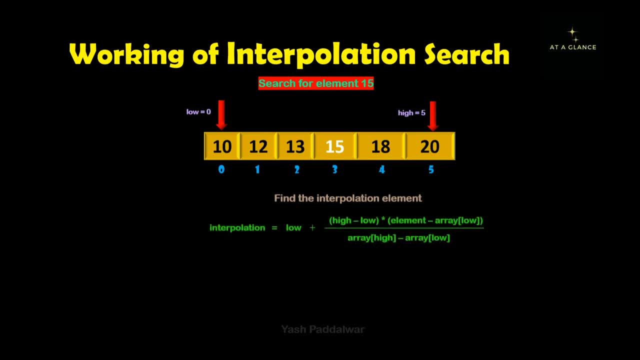 Now the next step is to find the interpolation element's position with the formula. So now we will put the values inside the formula. Low is 0.. High minus low is nothing but 5 minus 0. Element to be searched is 15.. 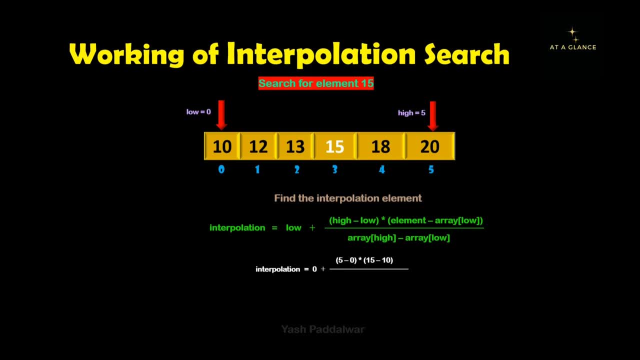 Minus the element which is located at 0th index is 10.. Divided by the element which is located at high index is 20 minus the element which is located as low index is 10.. Now solving the numerator, we get 5 into 5. divided by the denominator is nothing but 20 minus 10, which is 10.. 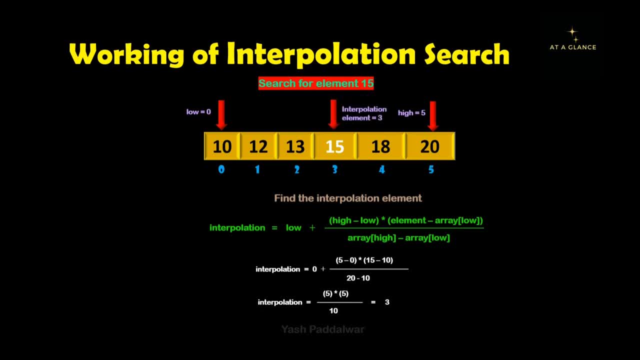 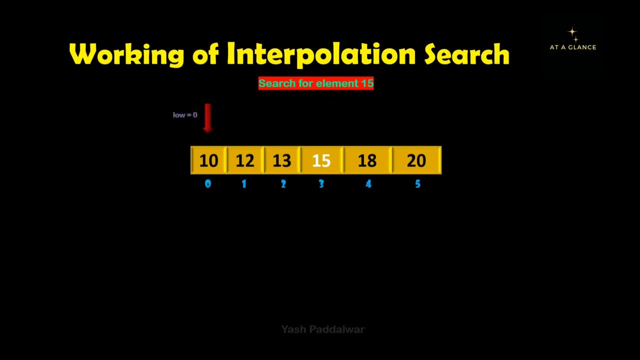 Now the entire calculation gives the output as 3.. So our interpolation element's position is 3.. Now, once you find the interpolation element's position, next step is to check the element which is located at the interpolation position is equal to the element to be searched or not. 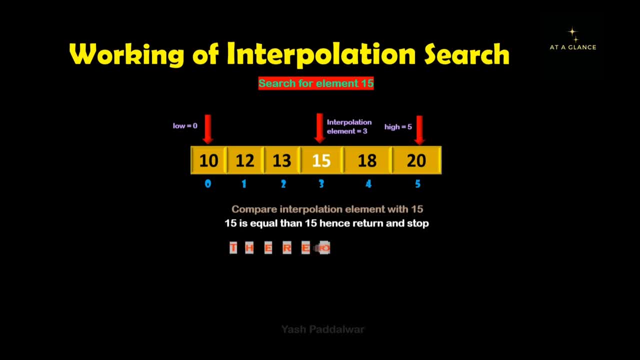 So clearly here we can see that 15 is equal to 15 and therefore we can say that the element is found at index position 3.. Now here we took an example of the data, which is uniformed, So therefore we have got the element to be searched in just one iteration. 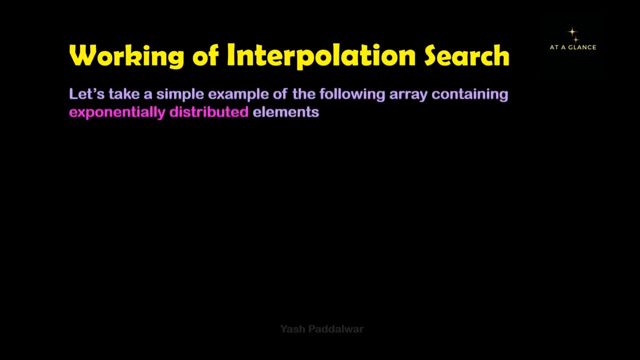 Hence, in this particular case, the interpolation search proves to be the best. Now let's take another example of an array which contains the data which is exponentially distributed. Now let's see how interpolation search works in this case. Let's say we need to search for the element 54 from the given array. 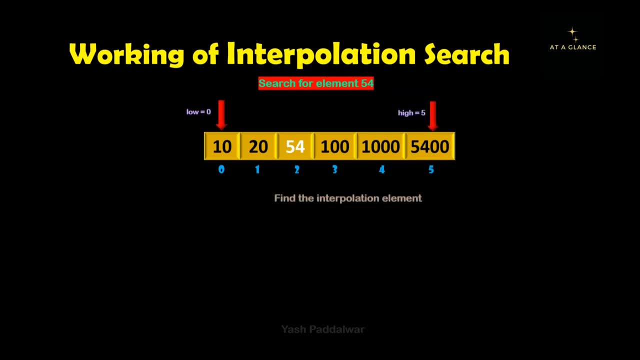 First step is to define the low position and high position. Low value will be 0 and high value will be 5.. Next step is to compute the interpolation element's position by the help of the formula. Let's plug in the values in the formula and therefore, after calculating, we get the answer as 0.. 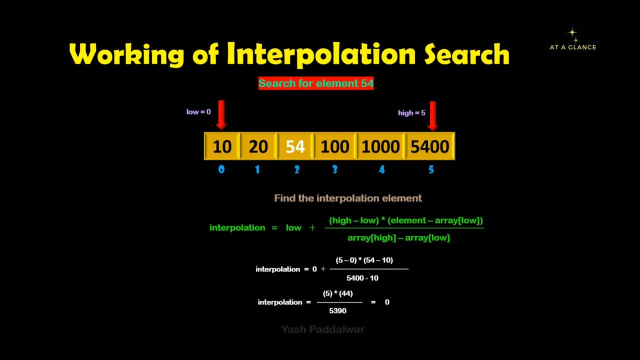 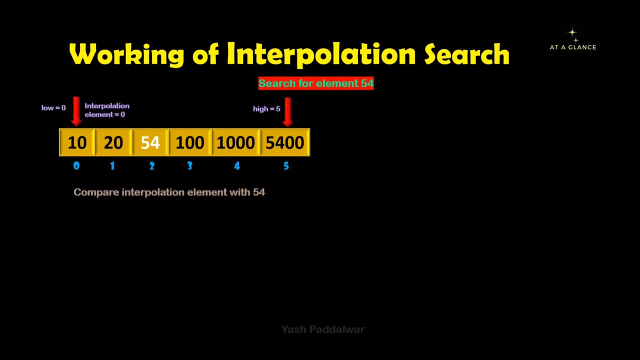 Therefore, in this case, the interpolation element's position is 0.. Next step is to compare the element which is located on the interpolation position with the element to be searched. Here, our element to be searched is 54 and the element which is located on the interpolation position is 10.. 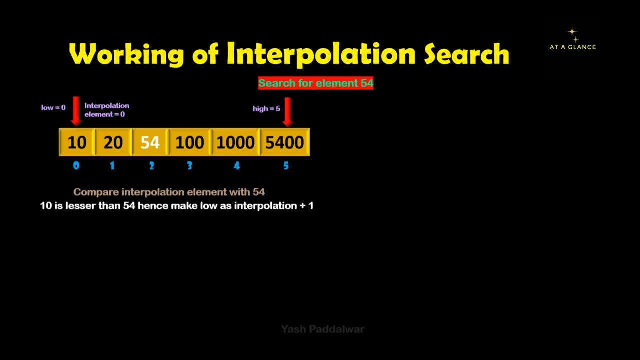 Clearly we can say 10 is not equal to 54, but we can say that 10 is lesser than 54. Therefore we will make low as interpolation plus 1.. Therefore our low now will be 0 plus 1, which is 1.. 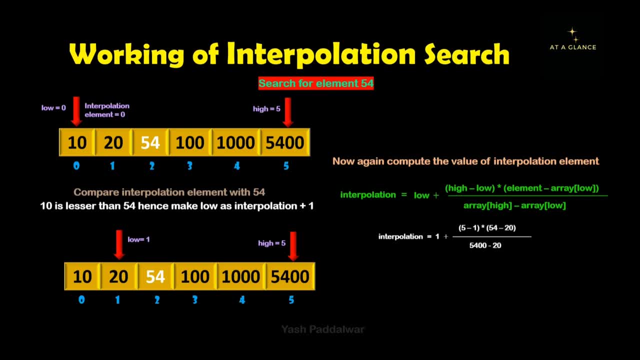 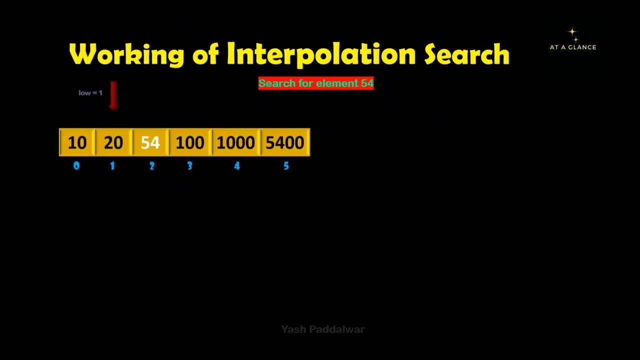 Now again compute the interpolation element's position with the help of the formula, Plugging in the values. we will get the interpolation element's position as 1.. Now again compare the interpolation element's position with the element to be searched. The element which is located at interpolation position is 20 and the element to be searched is 54..